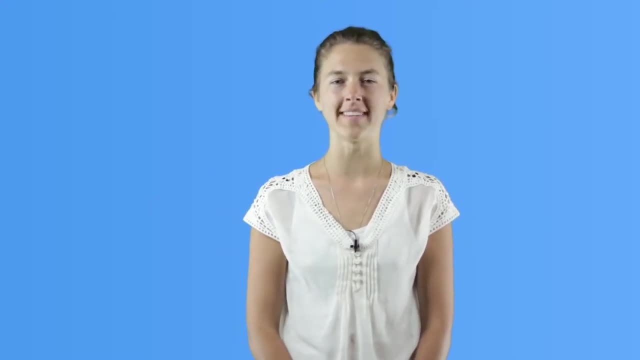 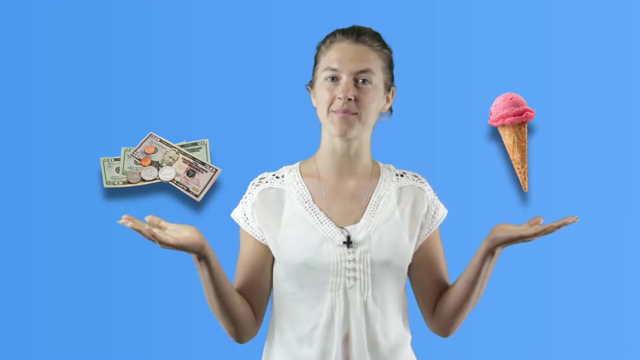 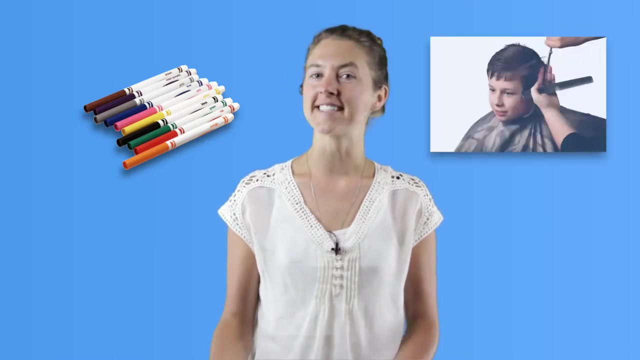 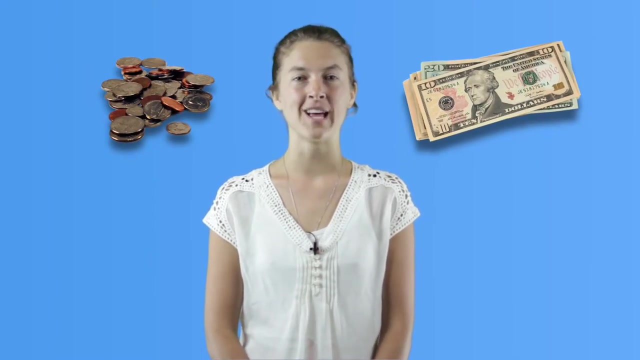 Hi, my name is Kylie and welcome to Counting Money 1, the value of money. Money is a way for us to exchange one thing for something else. We give money to get a product, like markers, or a service, like a haircut. In this video, you'll learn the value of coins and dollar bills. 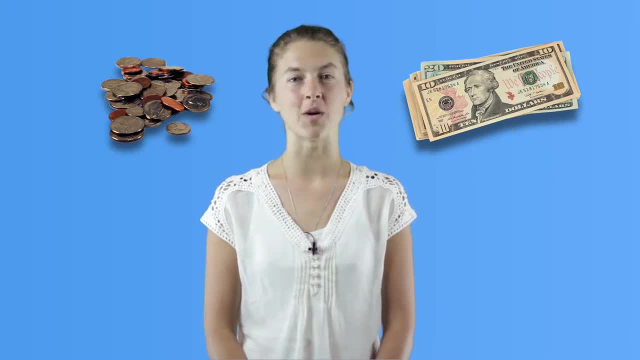 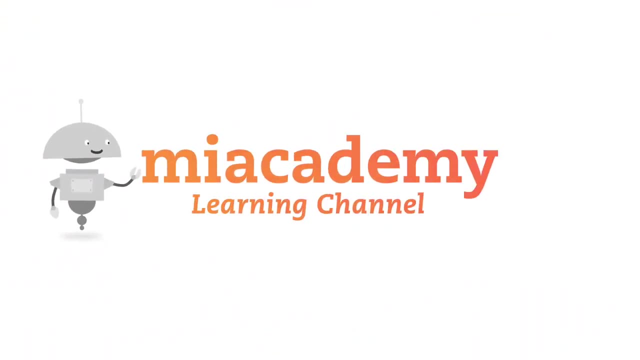 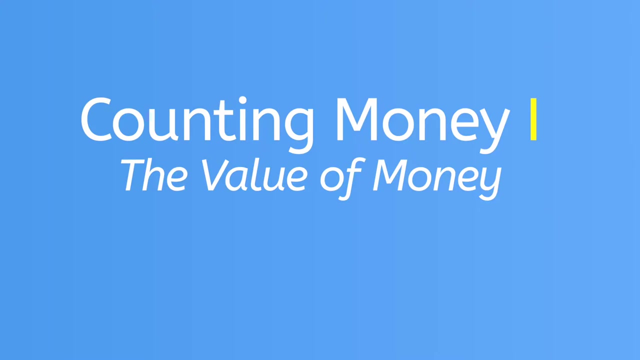 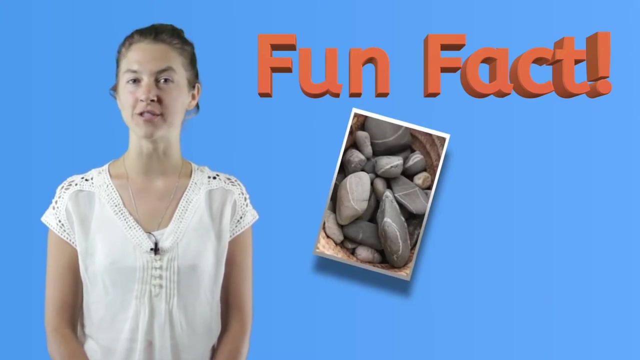 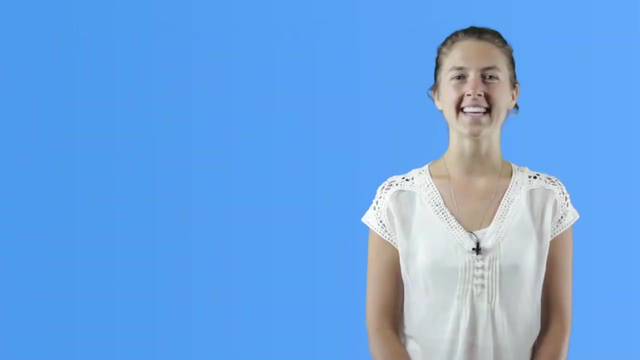 so that you can use money in exchange for something you want to buy. Did you know that before coins and bills, people traded stones, beads, feathers and other objects to get something they wanted? Whoa, Counting money is different from counting objects. 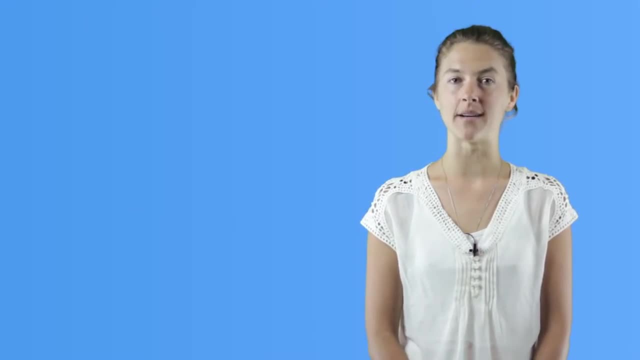 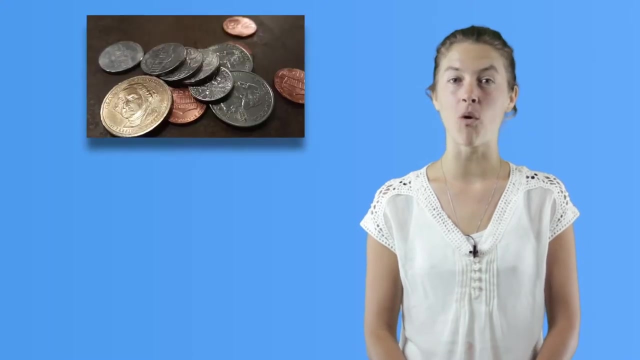 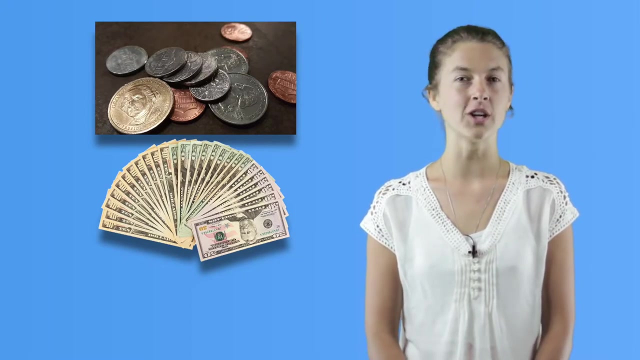 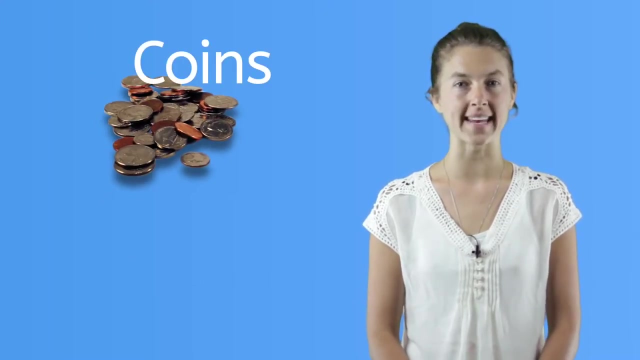 Money comes in denominations or set amounts. This means each type of coin or dollar bill has a special value. Let's look at the value of money more closely to understand what I mean. We're going to start with coins, which are small metal pieces of money. 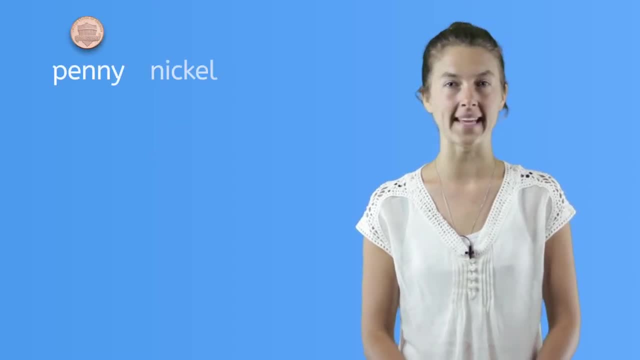 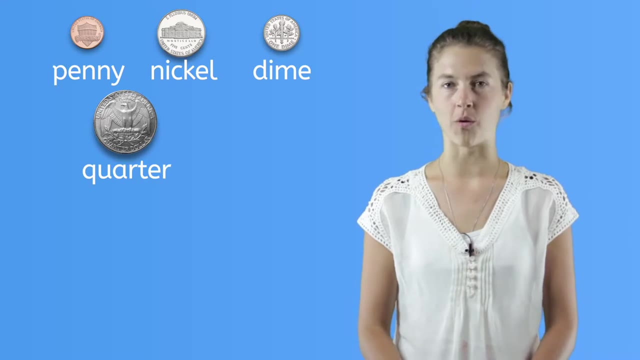 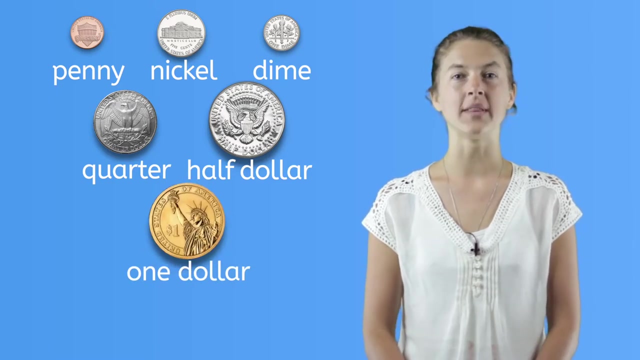 In the United States we have coins that represent one penny, five cents or a nickel, 10 cents or a dime and 25 cents or a quarter. We also have a half dollar coin and a gold-plated one dollar coin, but these are really rare and you may hardly see them. 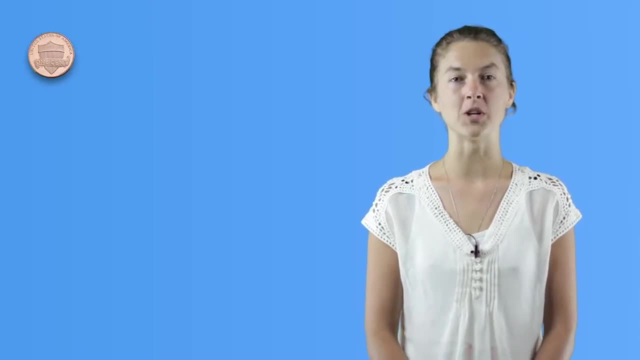 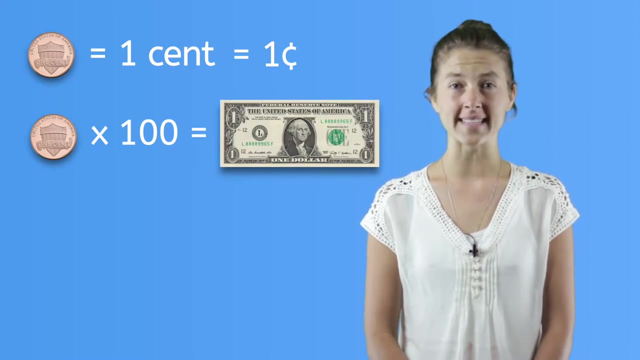 This is a penny. It is made of copper, which is why it is that color. A penny is worth one cent and this is the symbol for cent. There are 100 cents in one dollar. That means it takes 100 pennies to make one dollar. 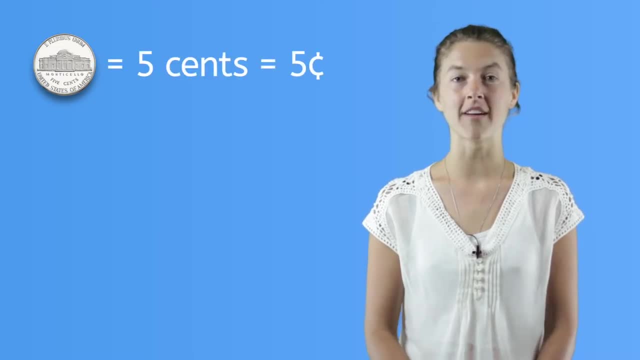 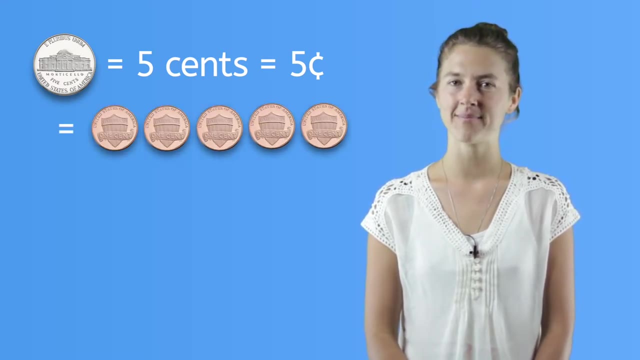 This is a nickel. A nickel is worth five cents, and five cents is the same as five pennies. A nickel is bigger than a penny in size and is silver instead of copper. When counting nickels, you'll count by fives, Five, ten, fifteen, twenty. 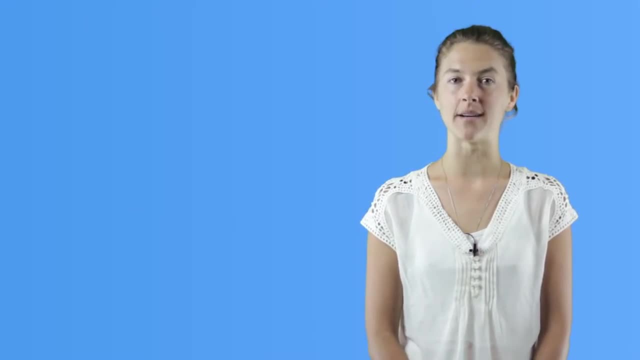 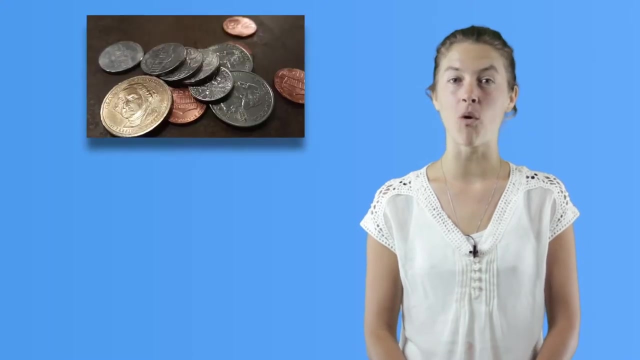 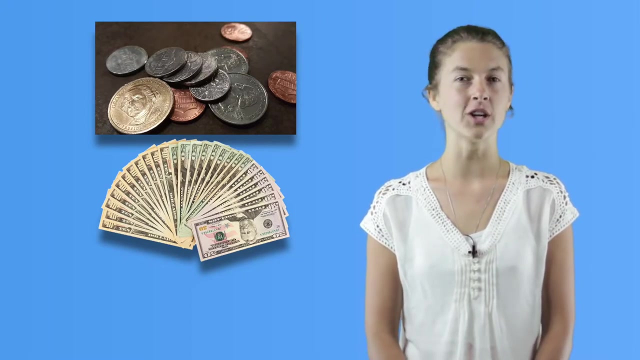 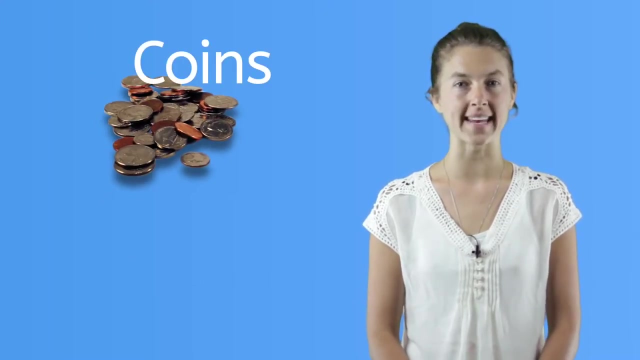 Money comes in denominations or set amounts. This means each type of coin or dollar bill has a special value. Let's look at the value of money more closely to understand what I mean. We're going to start with coins, which are small metal pieces of money. 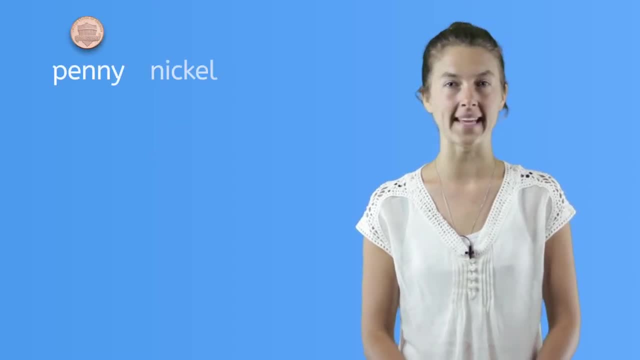 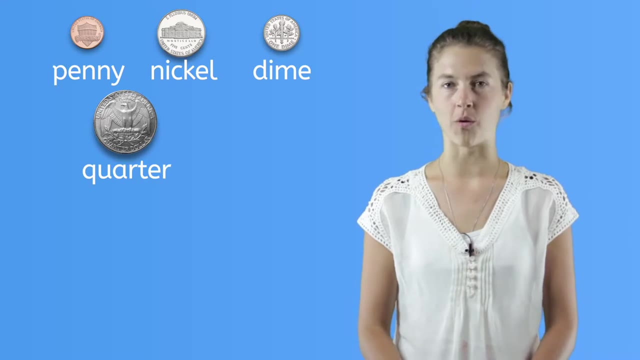 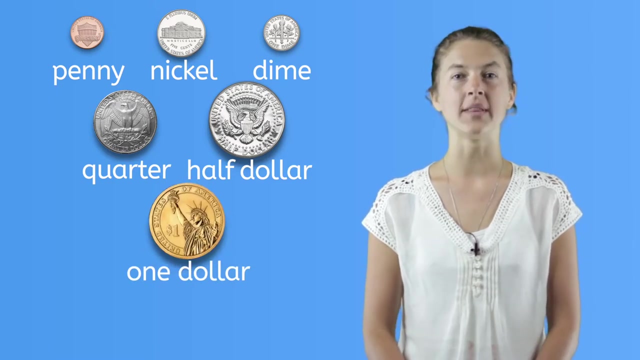 In the United States we have coins that represent one penny, five cents or a nickel, 10 cents or a dime and 25 cents or a quarter. We also have a half dollar coin and a gold-plated one dollar coin, but these are really rare and you may hardly see them. 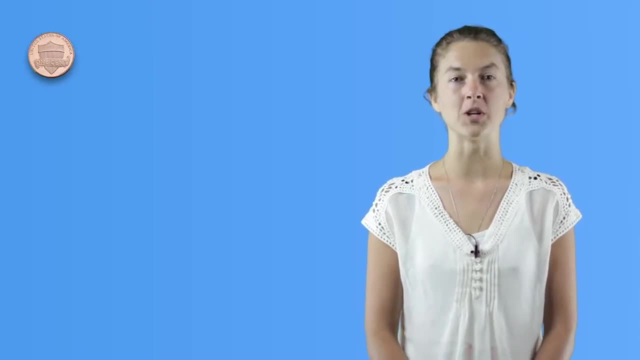 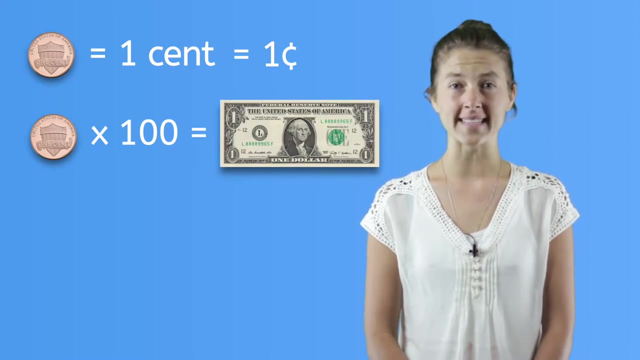 This is a penny. It is made of copper, which is why it is that color. A penny is worth one cent and this is the symbol for cent. There are 100 cents in one dollar. That means it takes 100 pennies to make one dollar. 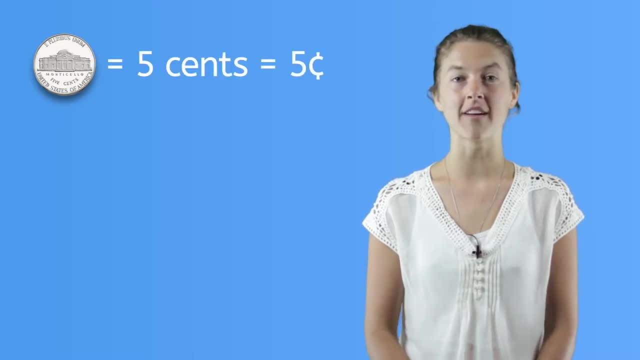 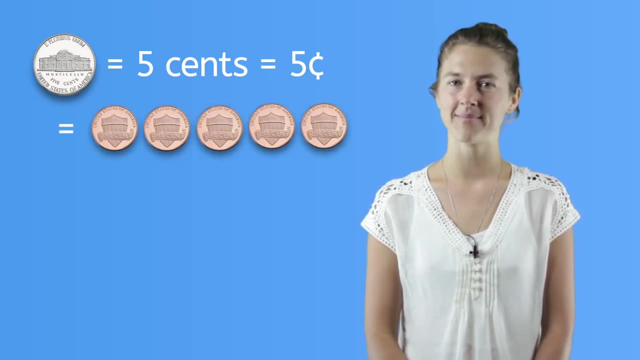 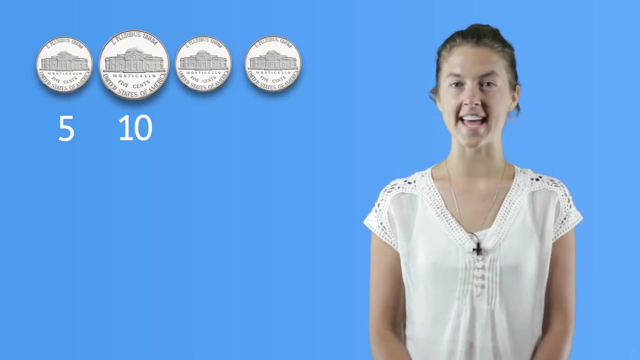 This is a nickel. A nickel is worth five cents, and five cents is the same as five pennies. A nickel is bigger than a penny in size and is silver instead of copper. When counting nickels, you'll count by fives: Five, 10,, 15,, 20.. This makes 20 cents. 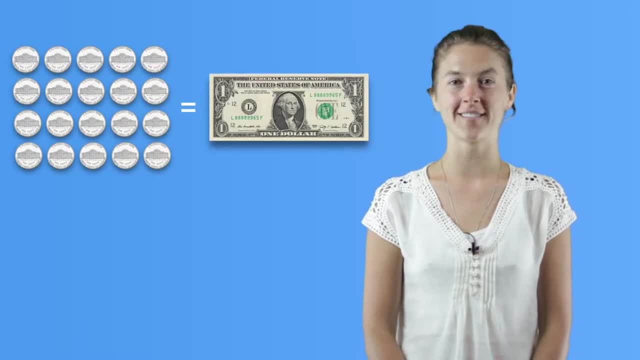 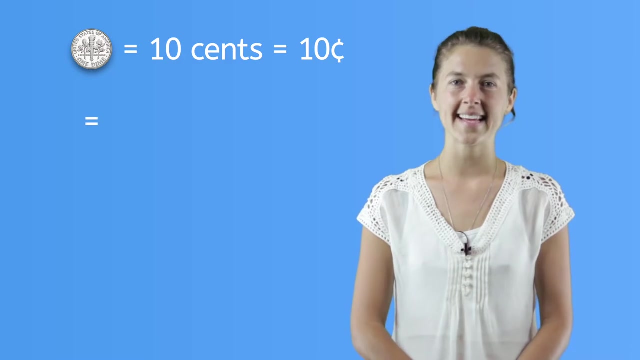 There are 20 nickels in one dollar. That means it takes 20 nickels to be worth the same as one dollar. This is a dime. A dime is worth 10 cents. 10 cents is the same as 10 pennies, but also the same as two nickels. 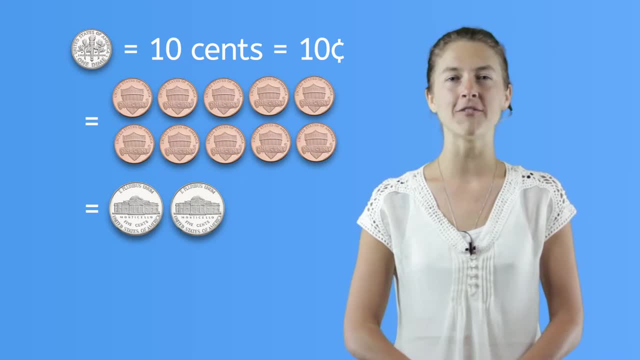 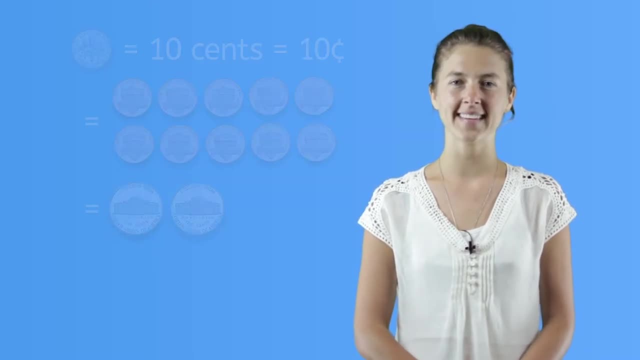 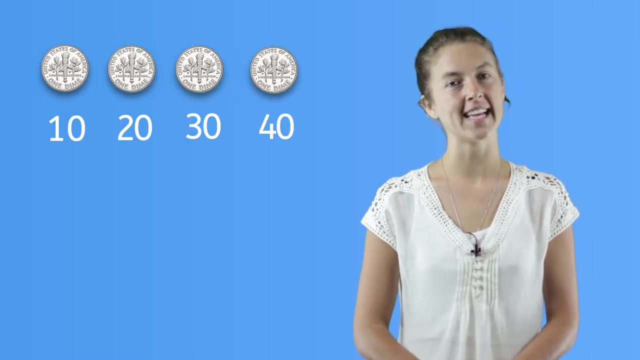 The dime is silver and quite small, but don't be fooled by its size. Even though it's small, it's actually worth more than a nickel. To count dimes, you'll count by tens: 10,, 20,, 30,, 40. This makes 40 cents. Time up in one dollar and a quarter. There are ten dimes in one dollar, So you'll need ten dimes to make one whole dollar. This is a quarter. A quarter is worth 25 cents To make the same value as a quarter. 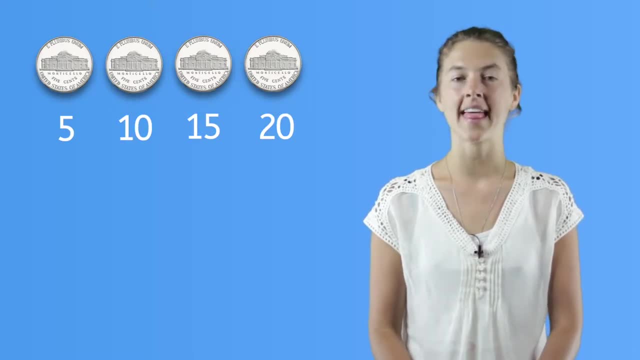 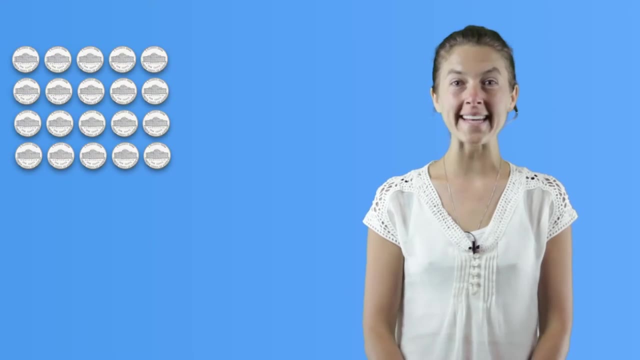 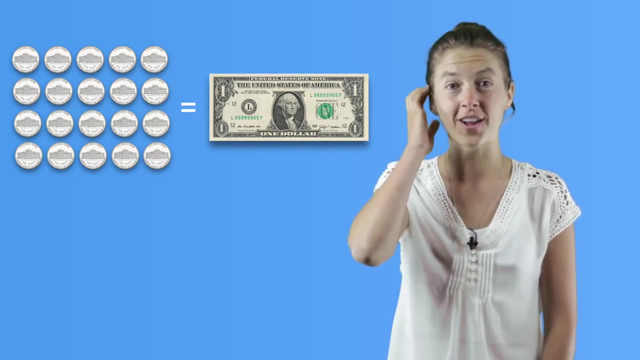 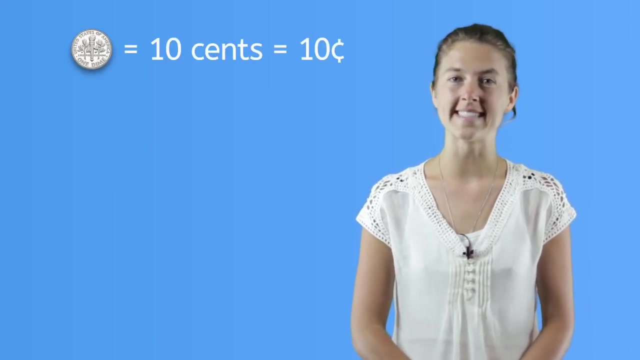 This makes 20 cents. There are 20 nickels in one dollar. That means it takes 20 nickels to be worth the same as one dollar. This is a dime. A dime is worth 10 cents. A dime is worth 10 cents. 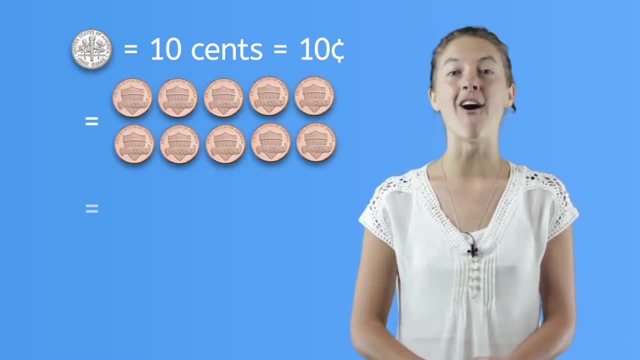 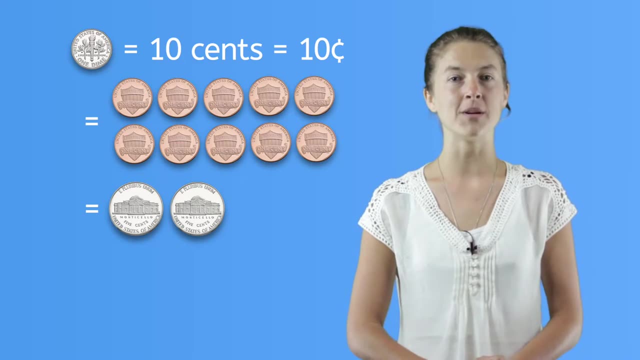 10 cents is the same as 10 pennies, but also the same as 2 nickels. The dime is silver and quite small, but don't be fooled by its size. Even though it's small, it's actually worth more than a nickel. 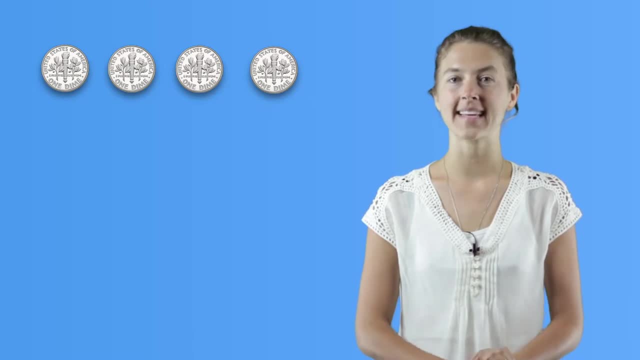 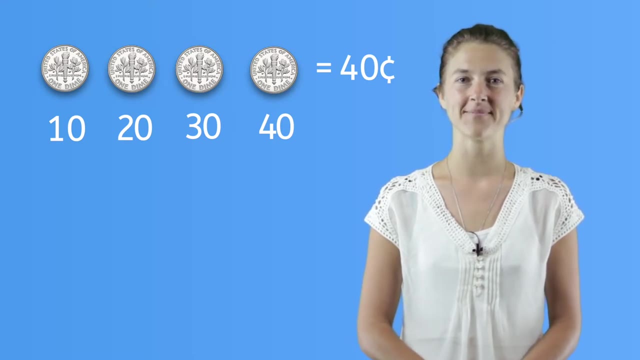 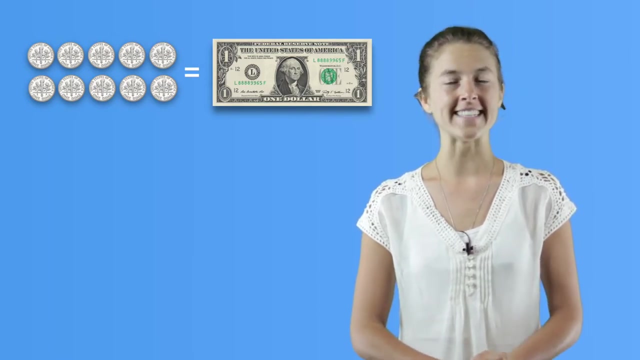 To count dimes you'll count by tens: 10,, 20,, 30,, 40. This makes 40 cents. There are 10 dimes in one dollar, So you'll need 10 dimes to make one whole dollar. 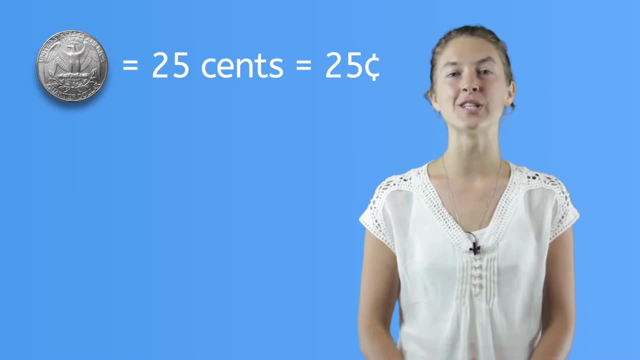 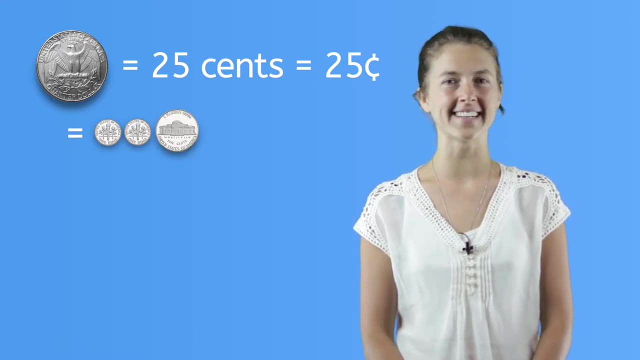 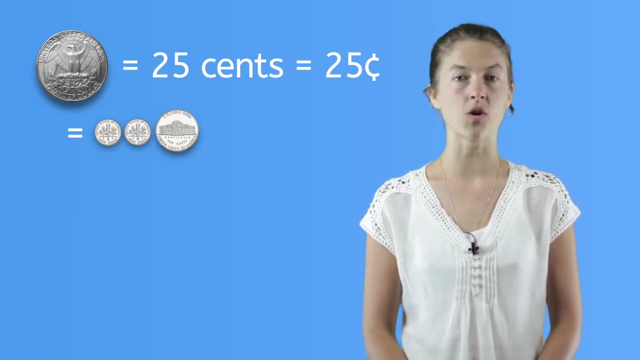 This is a quarter. A quarter is worth 25 cents. To make the same value as a quarter you would need 2 dimes plus a nickel. That's 25 cents. A quarter is larger in size than the other coins and it's silver. 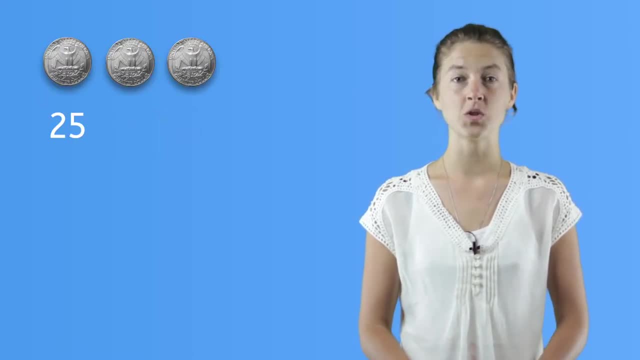 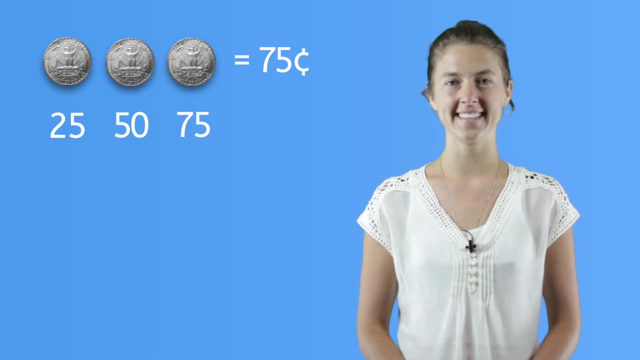 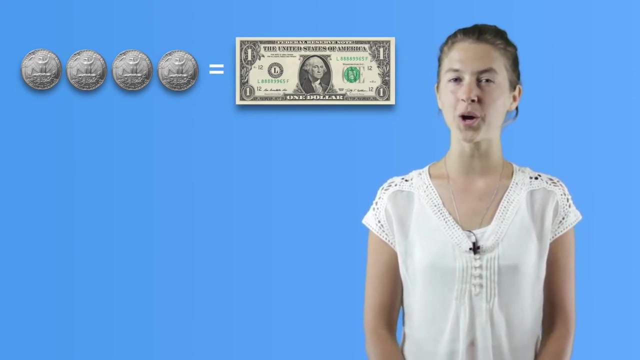 You'll count quarters by 25s: 25, 50, 75. You have 75 cents here. There are 4 quarters in a dollar. That means you'll need 4 quarters to have the same value as one dollar. 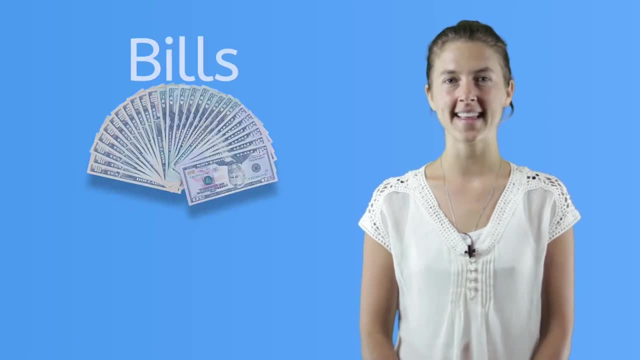 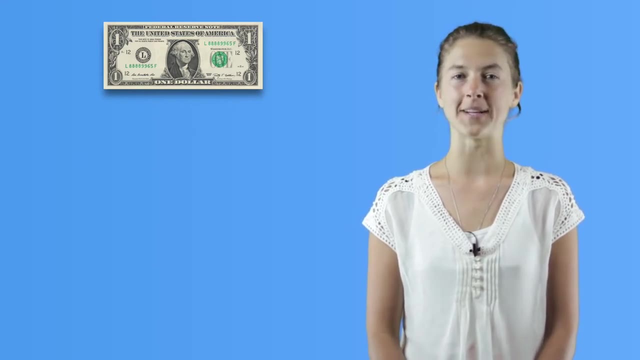 Paper money is known as dollar bills. This is one dollar bill. You'll count these as 1.. A one dollar bill is the same amount as 4 quarters, 10 dimes, 20 nickels or 100 pennies. 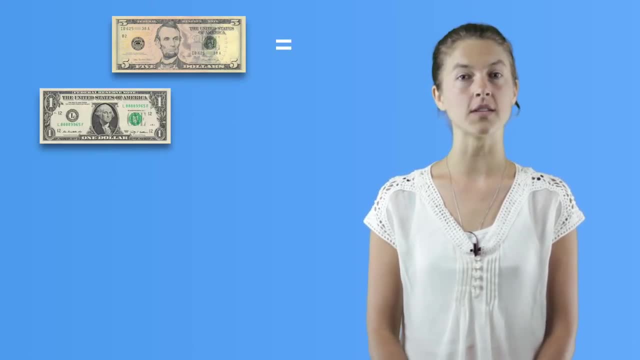 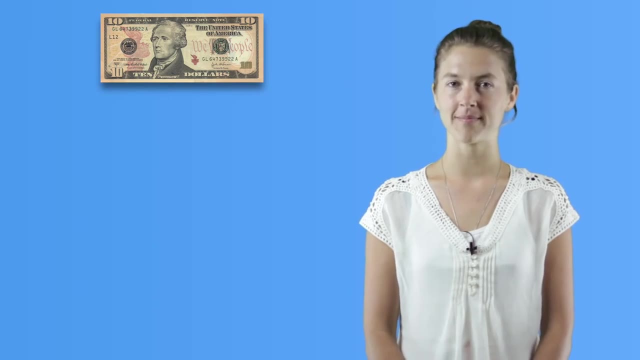 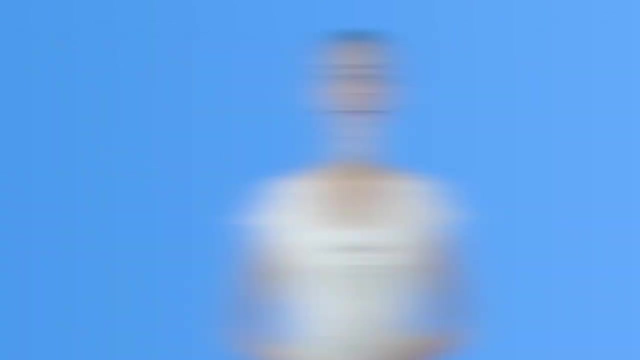 This is a 5 dollar bill. It equals 5 one dollar bills. This is a 10 dollar bill. It's the same as 10 one dollar bills or 2 5 dollar bills. This is a 20 dollar bill. 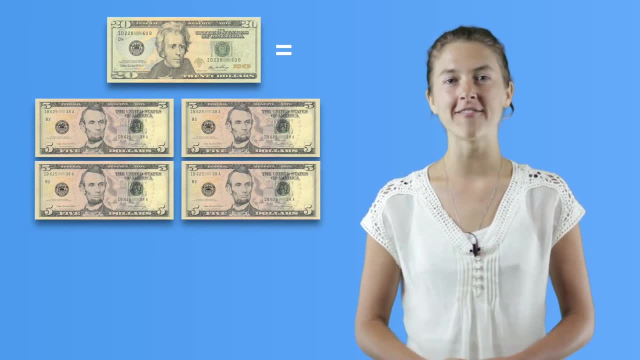 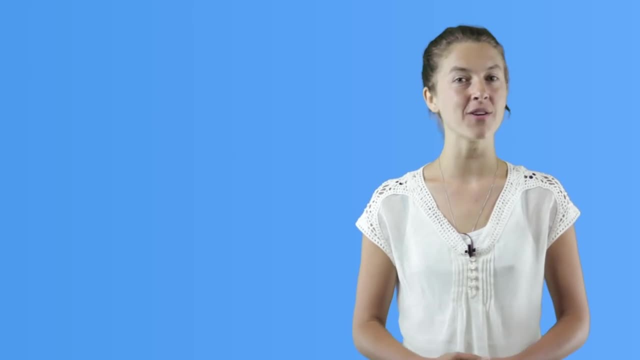 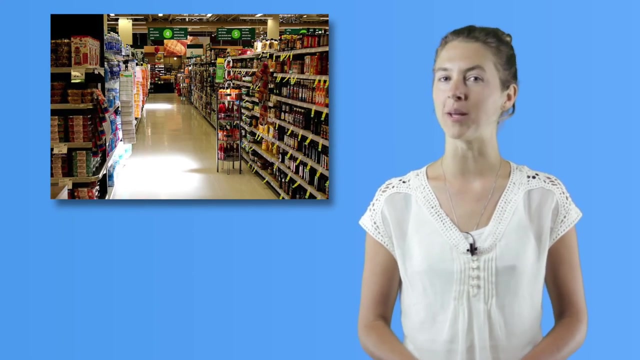 It's the same as 2 10 dollar bills, 4 5 dollar bills or 20 one dollar bills. You can now understand the value of money you receive as gifts or as an allowance. You can practice some more when you go shopping with your parents. 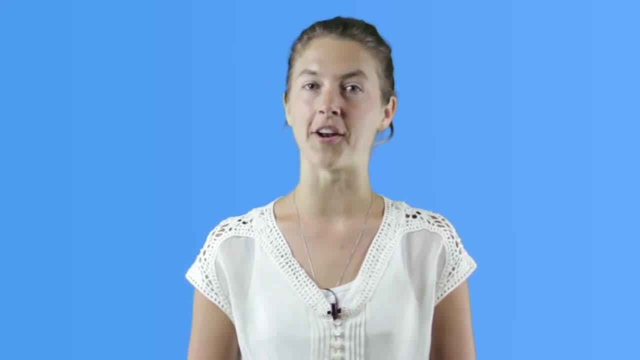 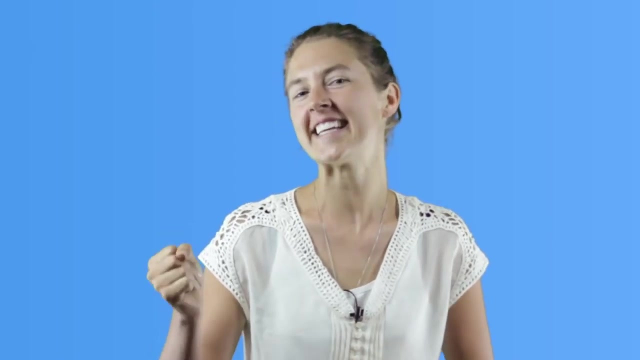 If you want to test your skills, try counting money on our fun online games and quizzes, And remember to always be clever Cha-ching. 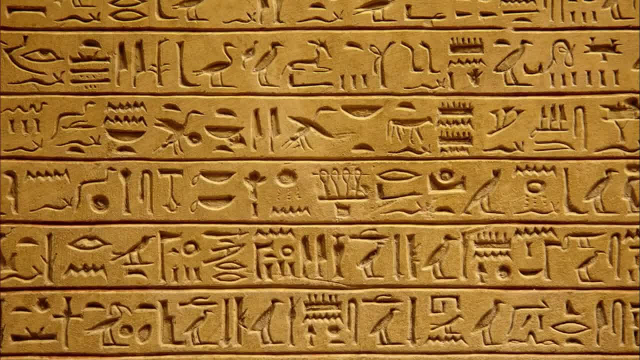 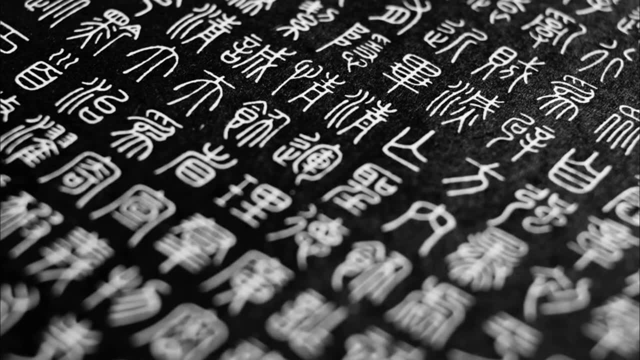 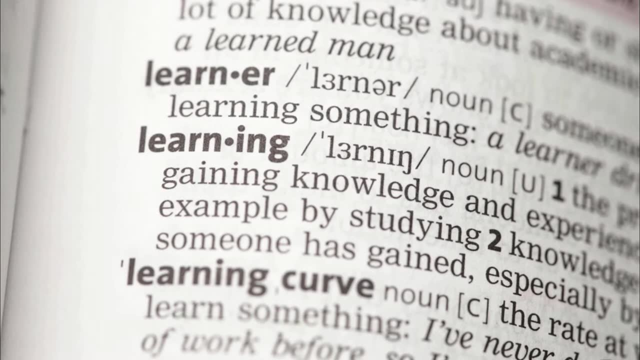 The earliest forms of written language were visual. They were symbology: The image, the picture represented the concepts being communicated. As communications evolved, our written language became more nuanced to communicate more complex ideas, But that hasn't helped us when communicating numbers. We can actually parse numbers much. 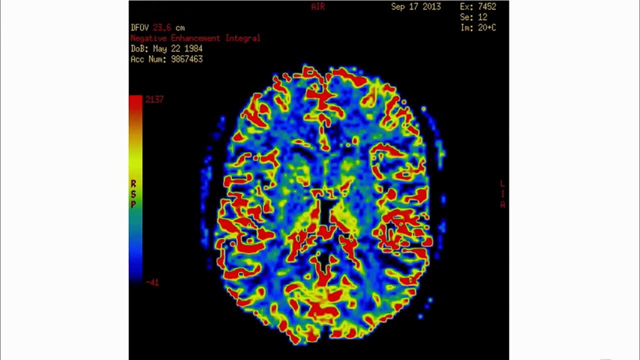 more quickly and easily in visual form, not text. Why is that? There are a number of reasons. One thing is that 30-50% of our brain is devoted to visual processing and 70% of our sensory receptors are in our eyes. It's also been shown that it takes a tenth of a second to make sense. 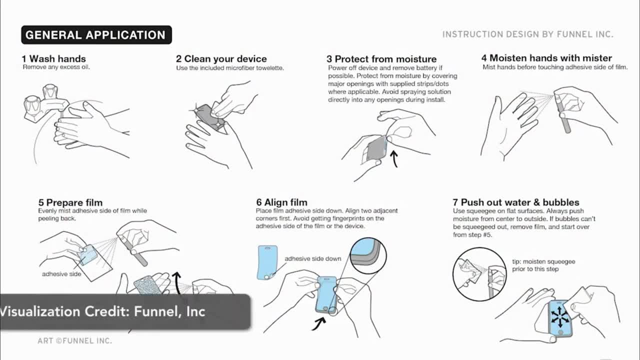 of a visual scene just at the glance of an eye. It's also been shown that you have 323% better performance on tasks when you learn them accompanied by images versus just text. There's also something known as the picture superiority effect that you'll remember 60% of. 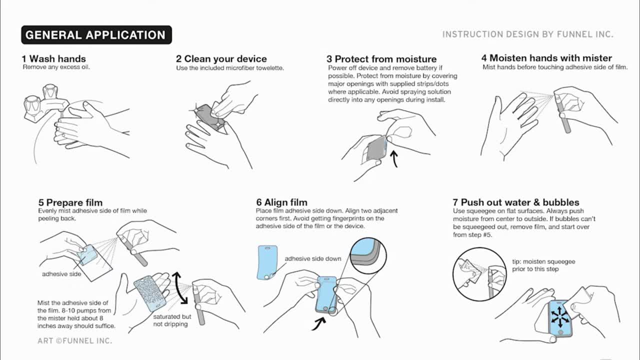 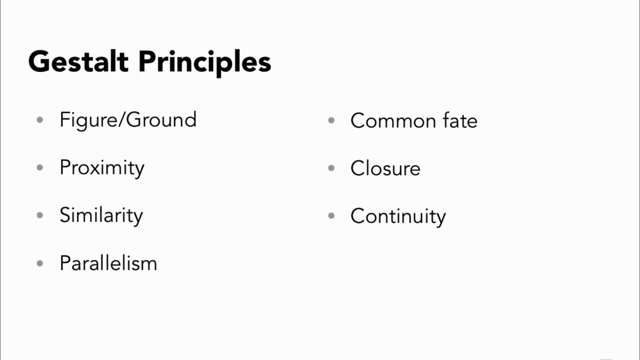 something when you learn it with imagery versus 6% without, and this effect increases with age. There's also something called gestalt psychology, and these gestalt principles have a deep effect in how we perceive visual information. This helps immensely with data visualization to 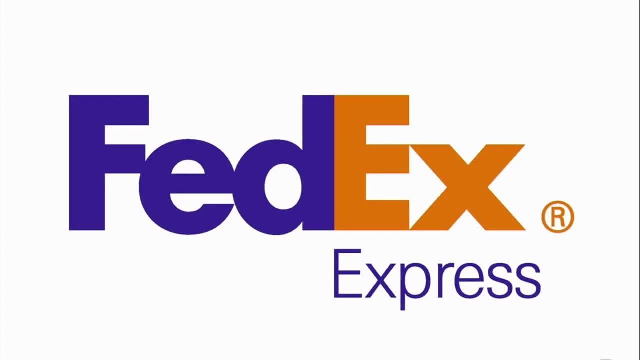 understand how it works. The first one is called figure ground. It's most often used in logo design, for instance. here you have the FedEx logo, one of the more famous examples of the use of figure ground. You have the mark FedEx, the letters in the foreground and in the background the negative. 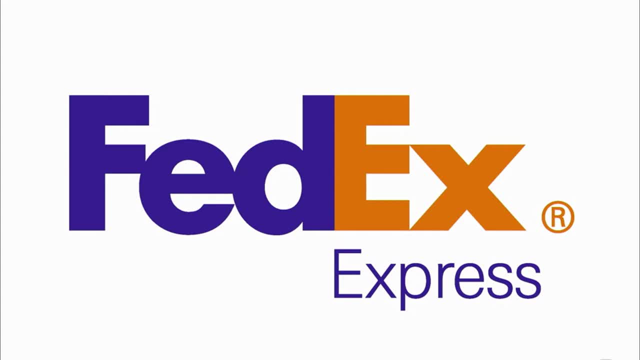 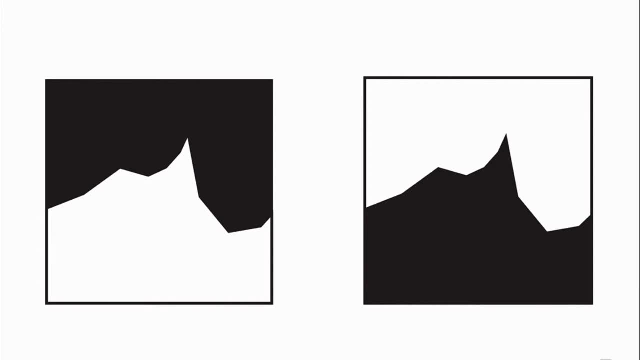 space you have that arrow, that white arrow, subliminal effect characterizing motion, which, of course, is what FedEx is all about. In data visualization, figure ground is the least actively used aspect of visual perception, but it is important to understand What's interesting is.